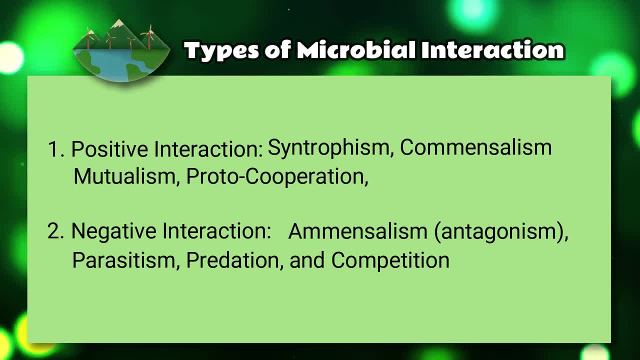 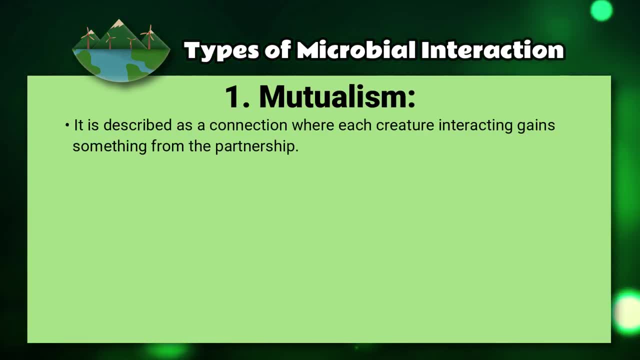 whereas negative includes amensalism, parasitism, predation and competition. First let's learn about mutualism. Mutualism is described as a connection where each creature interacting gains something from their partnership. Mutualists and hosts are physiologically obligated to one another in 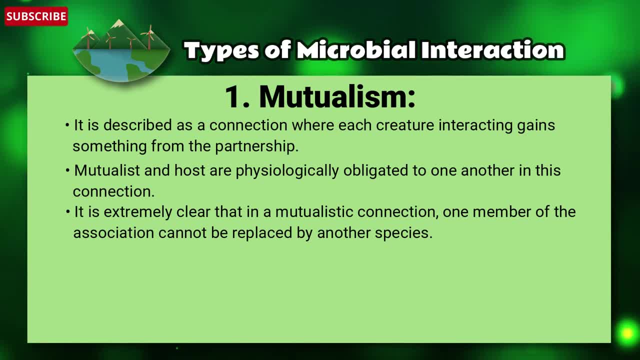 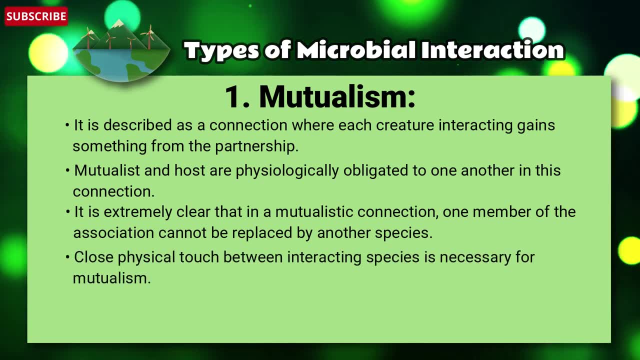 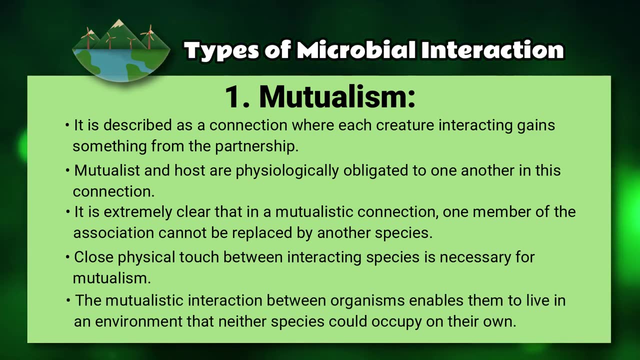 this connection, It is extremely clear that in a mutualistic condition, one member of the association cannot be replaced by another species. Close physical touch between the interacting species is necessary for mutualism. The mutualistic interaction between organisms can enable them to live in an environment that neither species could occupy on their own. 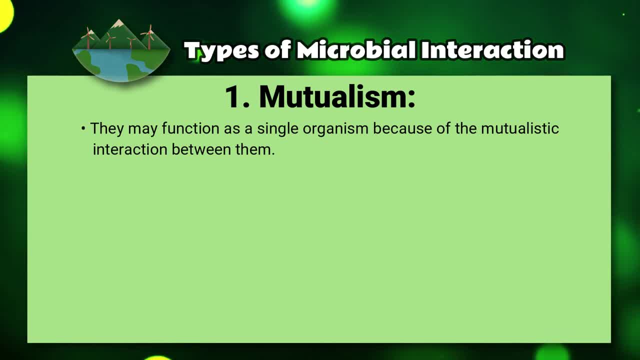 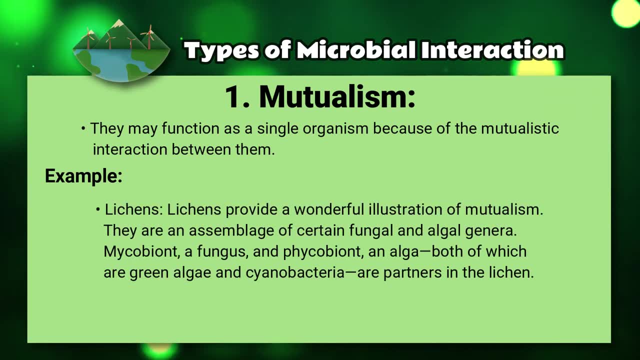 They may function as a single organism because of the mutualistic interaction between them. One example is lichens. Lichens provide a wonderful illustration of mutualism. They are an assemblage of certain fungal and algal genera- mycobiotes, a fungus. 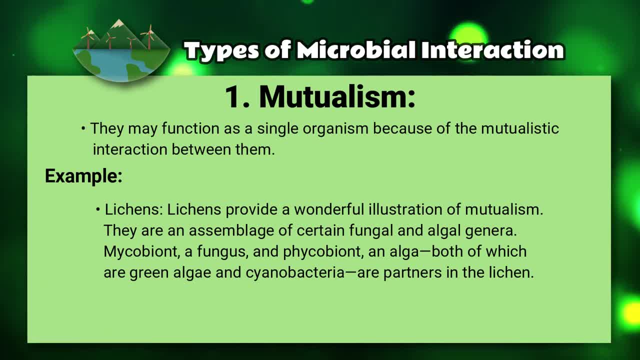 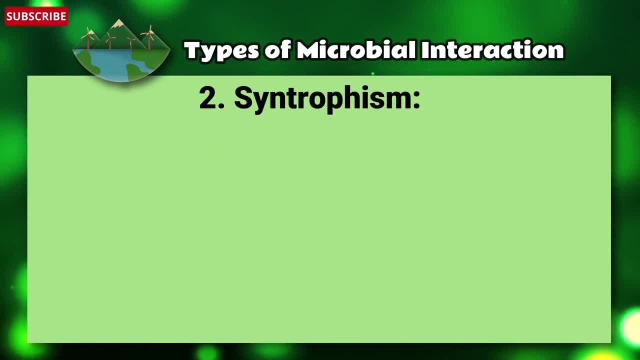 and a. phycobiotes and alga, both of which are green algae- and cyanobacteria are partners in the lichen. Don't forget to subscribe to my channel 2.. Scientrophism: It is a relationship in which one organism's development is either influenced by or enhanced. 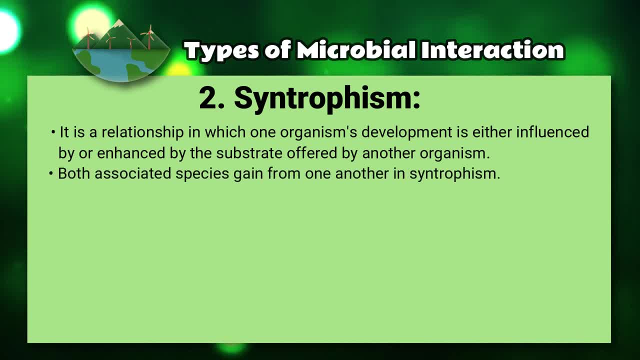 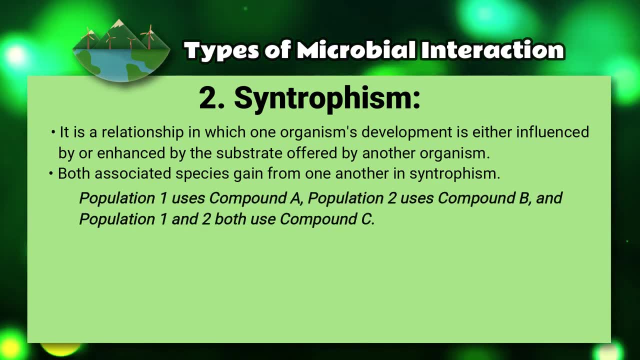 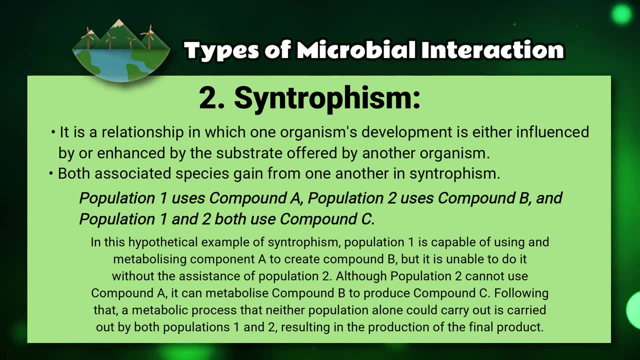 by the substrate offered by another organism. Both associated species gain from one another in scientrophism, Like population 1 uses compound A, population 2 uses compound B, and population 1 and 2 both uses compound C, As you heard in this hypothetical example. 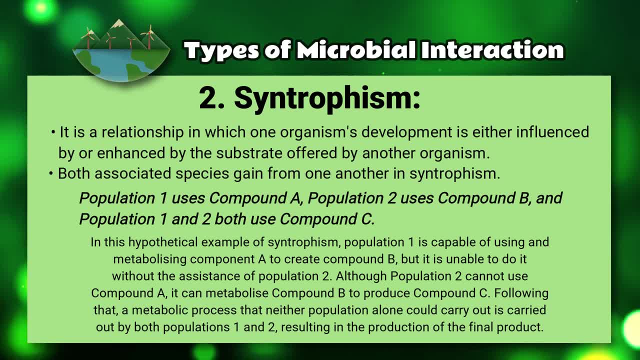 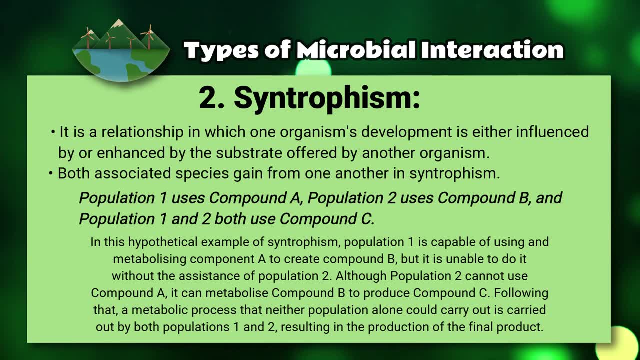 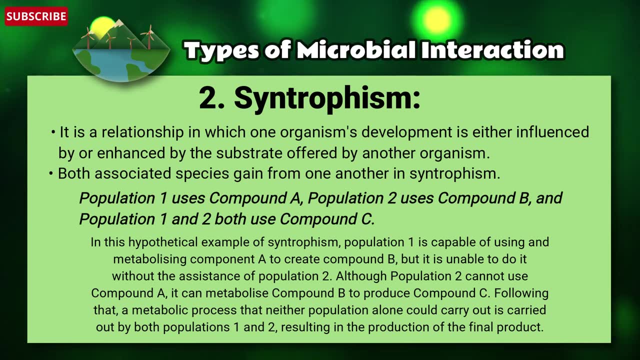 of scientrophism, population 1 is capable of using and metabolizing component A to create compound B, but it is unable to do it without the assistance of population 2.. Although population 2 cannot use compound A, it can metabolize compound B to produce compound C. 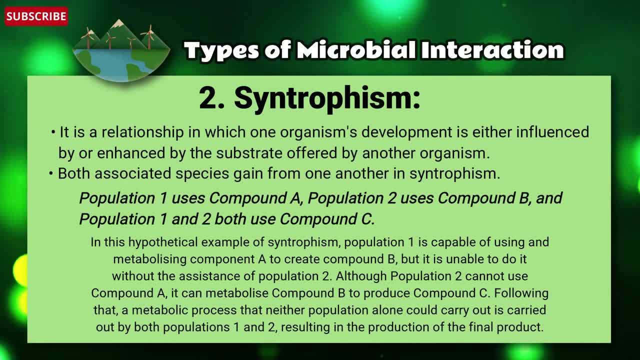 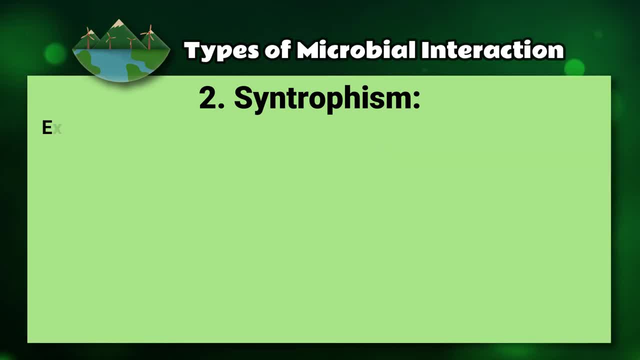 Following that, a metabolic process that neither population alone could carry out is carried out by both population 1 and 2, resulting in the production of the final product. 3. Metabolism: Two examples of this are methanogenic ecosystem in a sludge digester. 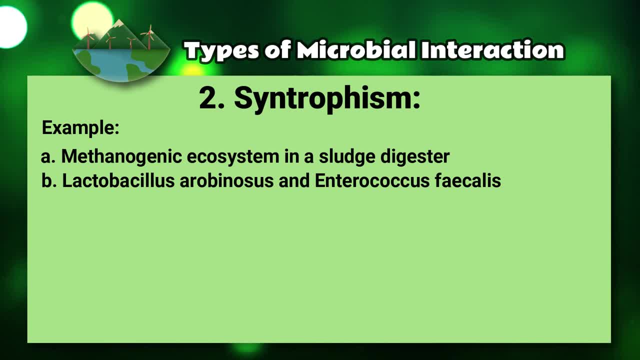 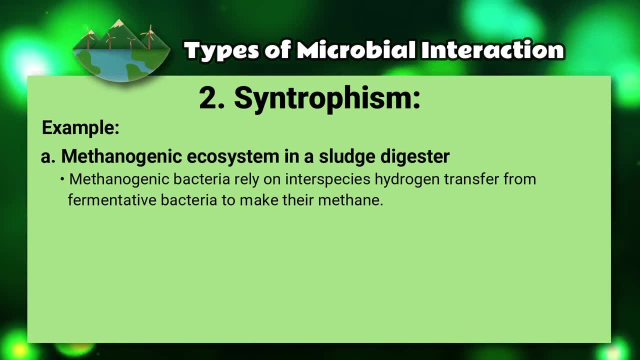 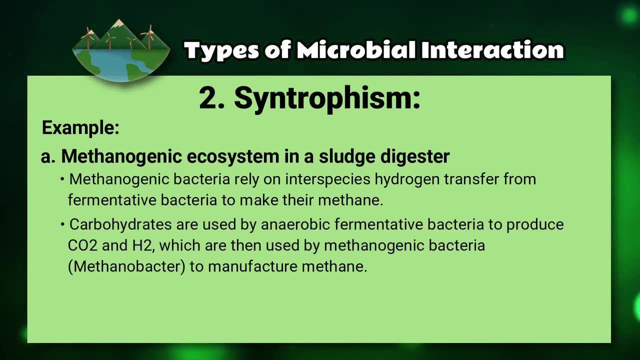 Lactobacillus aerobinosis and Enterococcus faecalis. Methanogenic bacteria rely on interspecies hydrogen transfer from the fermentative bacteria to make their methane. Carbohydrates are used by anaerobic fermentative bacteria to produce carbon. 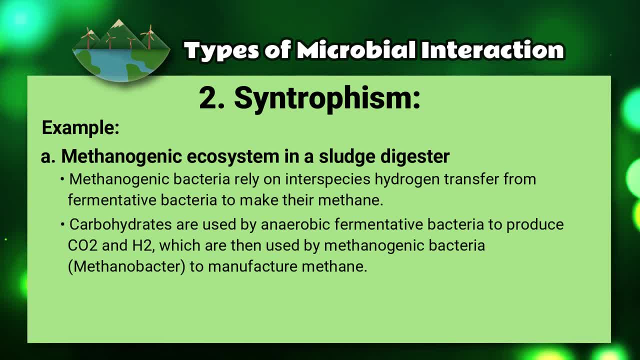 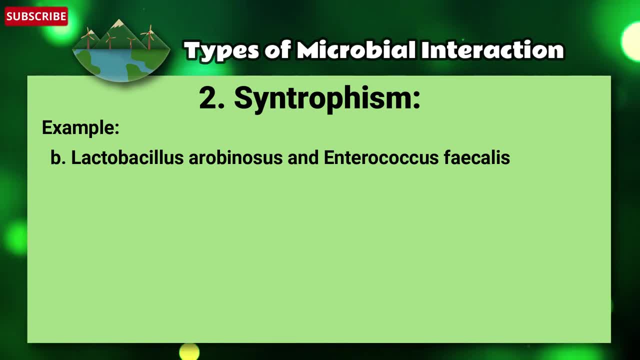 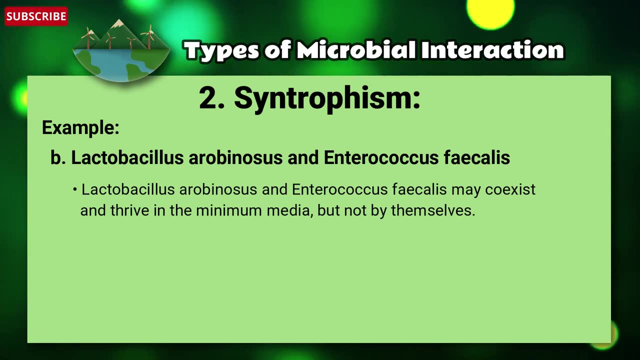 and H2, which are then used by methogenic bacteria to manufacture methane, Whereas in the other example, Lactobacillus aerobinensis and Enterococcus faecalis may coexist and thrive in the minimum media, but not by themselves. 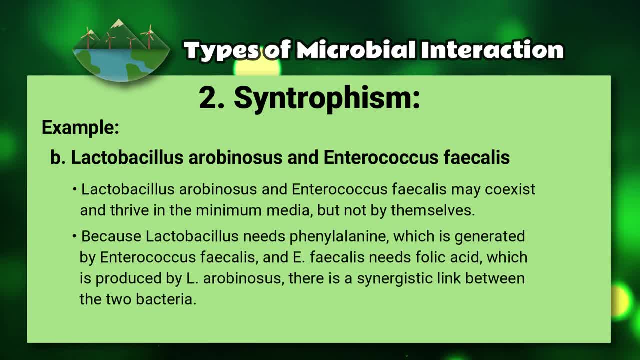 Because Lactobacillus needs phenylalanine, which is generated by Enterococcus faecalis, and Enterococcus faecalis needs folic acid, which is produced by Lactobacillus aerobinensis. there is a synaptic link between the two bacteria. 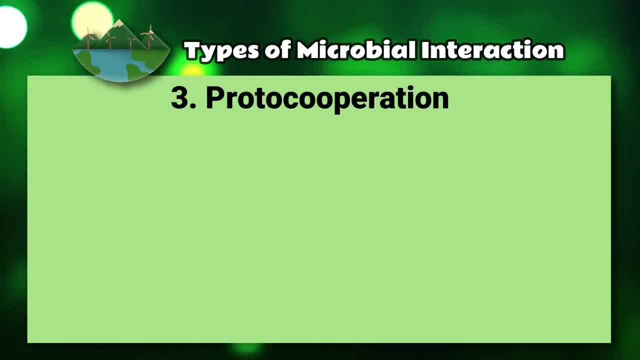 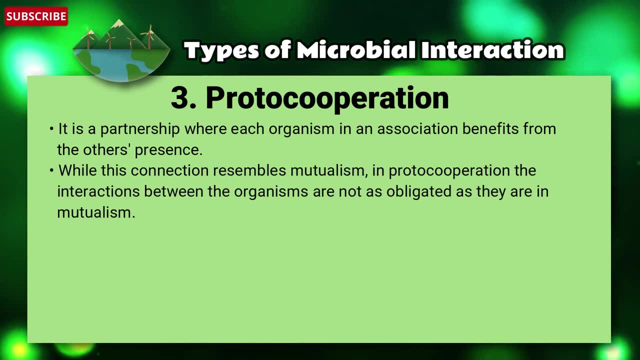 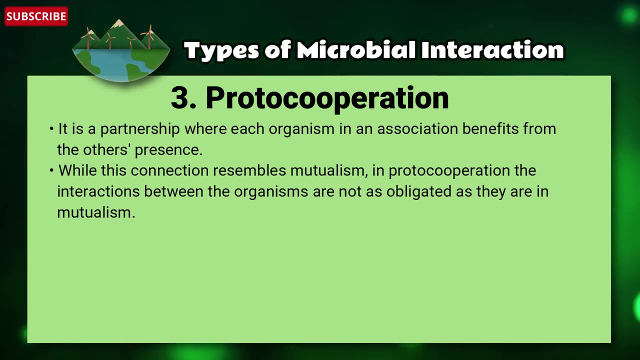 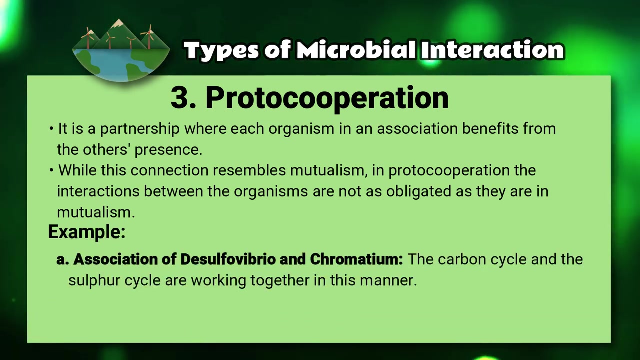 3. Proto-cooperation. It is a partnership where each organism in an association benefits from others' presence. While this connection resembles mutualism, in proto-cooperation the interactions between the organisms are not as obligated as they are. Examples are: 1. Association of desulfovibrio and chromatim. 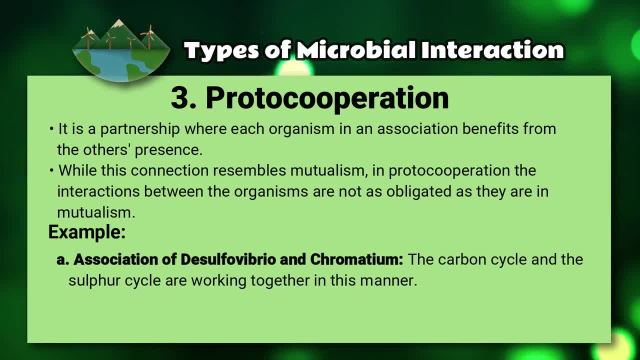 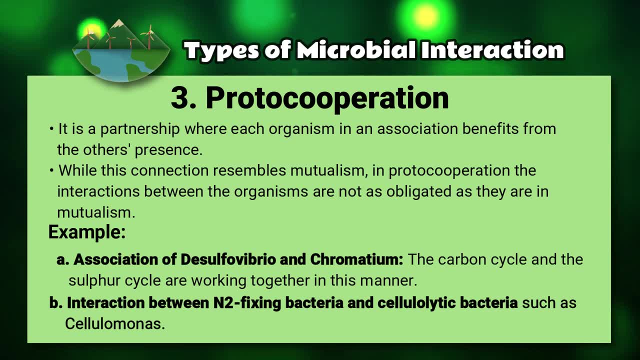 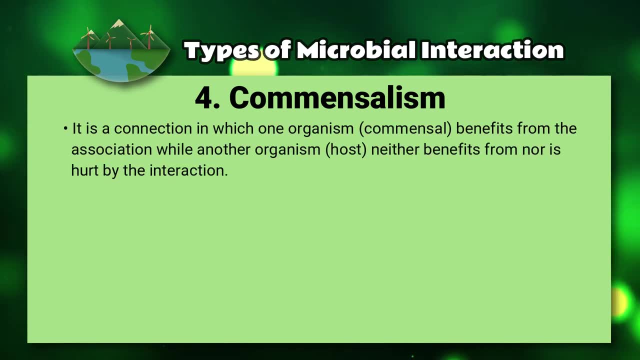 The carbon cycle and the sulfur cycle are working together in this manner. 2. Interaction between nitrogen-fixing bacteria and cellulolytic bacteria, such as cellulomonas. 4. Commensalism: It is a connection in which one organism, commensal, benefits from the association. 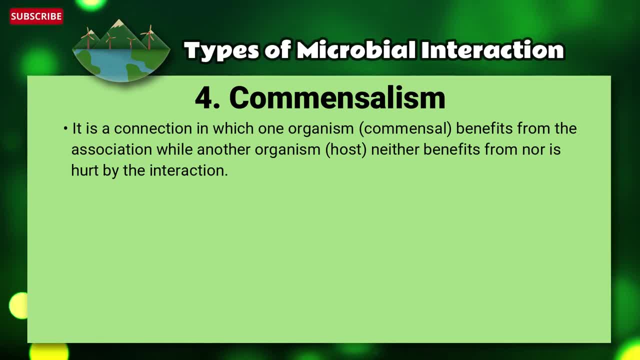 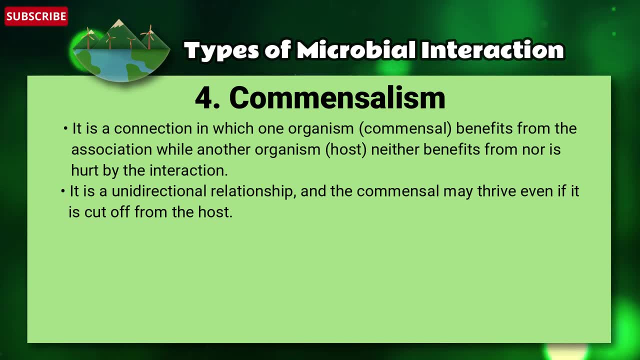 while another organism, homo, benefits, The host neither benefits from nor is hurt by the interaction. It is a unidirectional relationship and the commensal may strive even if it is cut off from the host. Examples of commensalism are: 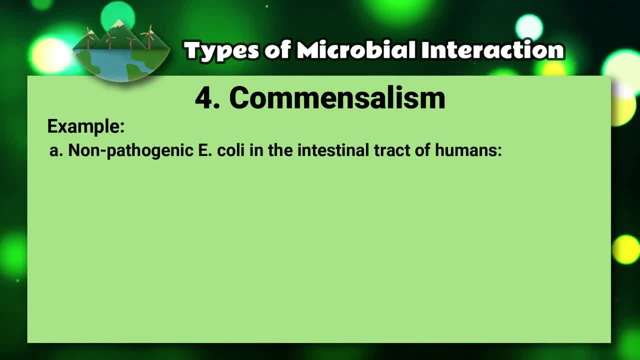 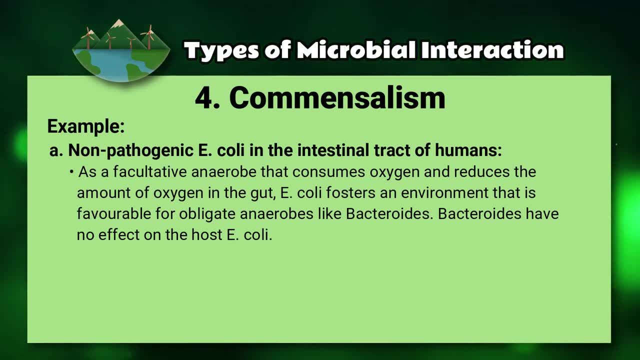 1. Non-pathogenic E coli in the intestinal tract of humans. As a feculative anaerobe that consumes oxygen and reduces the amount of oxygen in the gut, E coli fosters an environment that is favorable for obligate anaerobes like bacteroids. 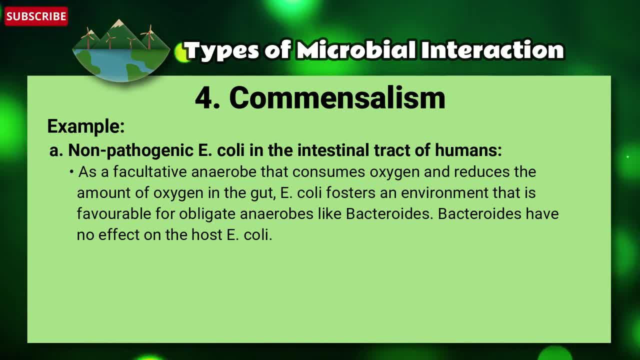 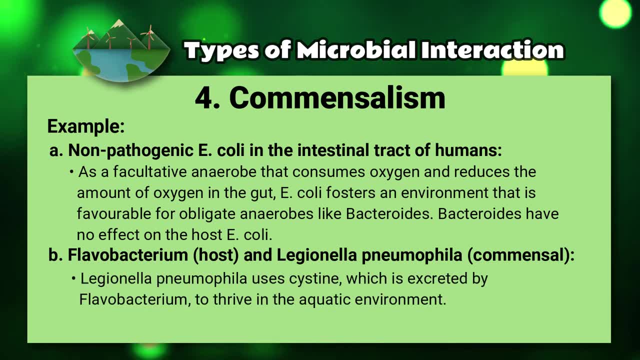 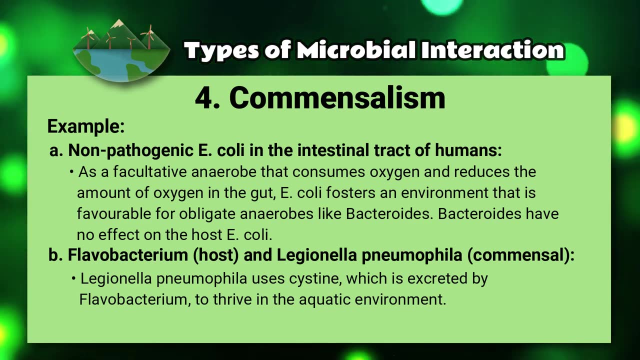 Bacteroids have no effect on the host E coli. 2. Flavobacterium host in N nemophila. commensal N nemophila use cytine which is extracted by flavobacterium to strive in the aquatic environment. 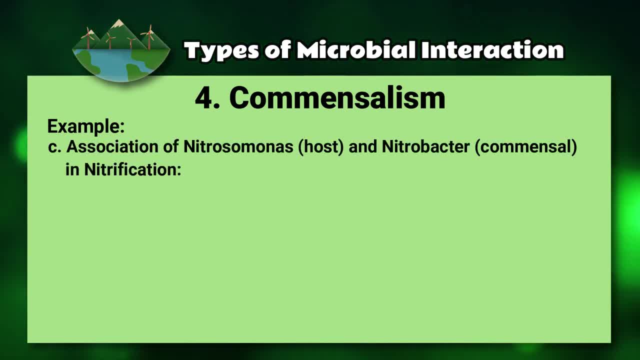 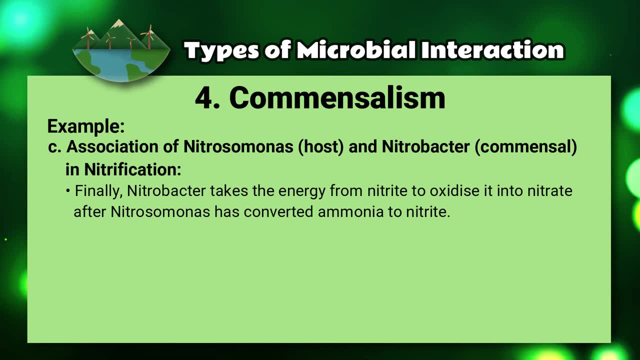 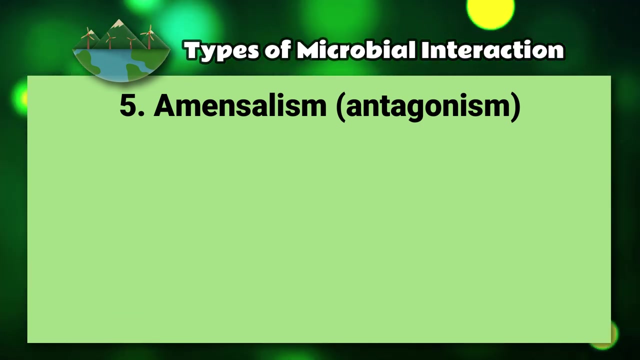 3. Nitrosomonas host in nitrobacter commensal in nitrification. Finally, nitrobacter takes the energy from nitrate to oxidize it into nitrate, after nitrosomonas has converted ammonia to nitrite. 5. Amensalism. 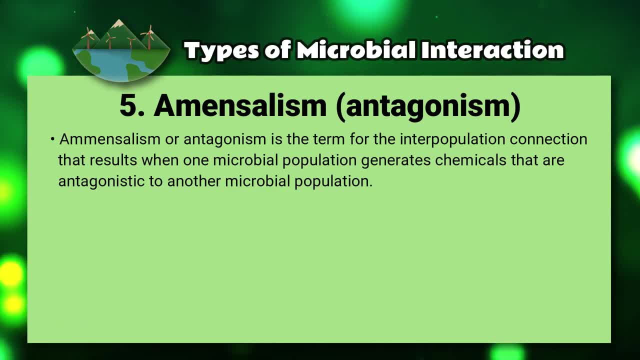 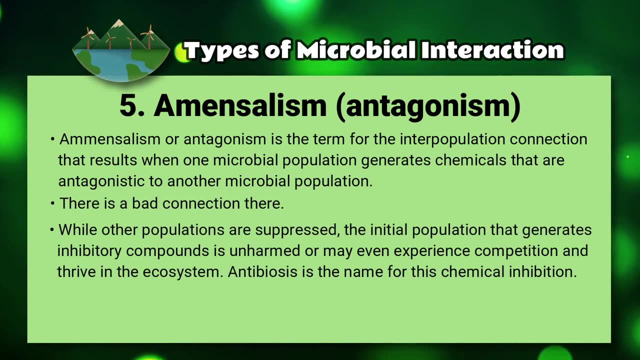 Amensalism or antagonism is a term for the interpopulation connection that results when one microbial population generates chemicals that are antagonistic to another microbial population. There is a bad connection there. While other populations are suppressed, the initial population that generates inhibitory compounds is unharmed. 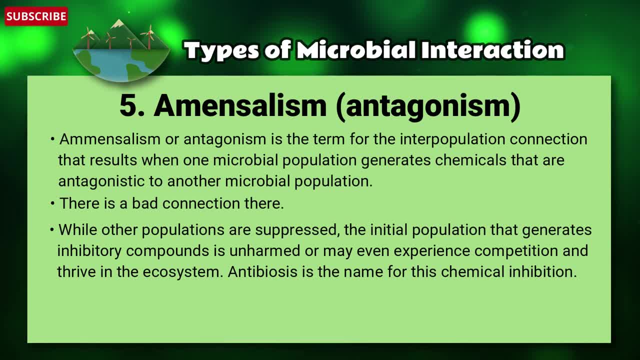 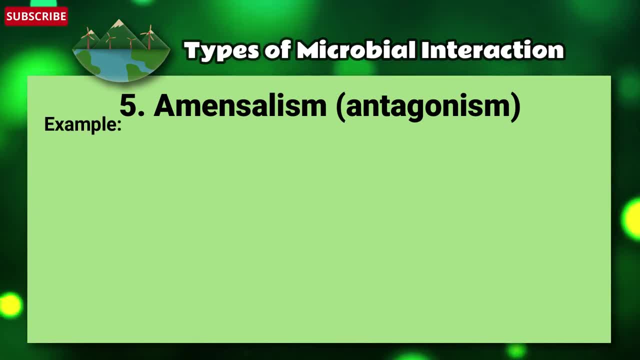 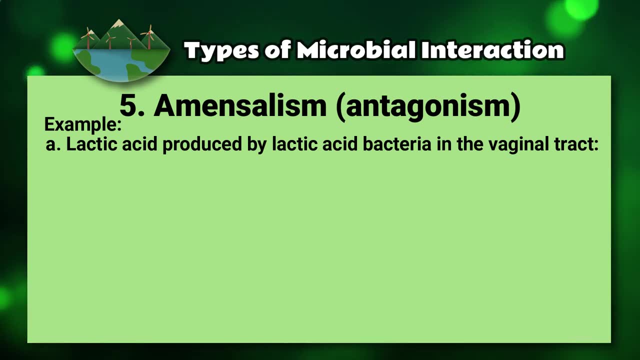 or may even experience competition that thrived in the ecosystem. Antibiosis is another name for this chemical inhibition. Examples of antagonism is: 1. Lactic acid produced by lactic acid bacteria in the gut. Lactic acid is produced by lactic acid bacteria in the vaginal tract. 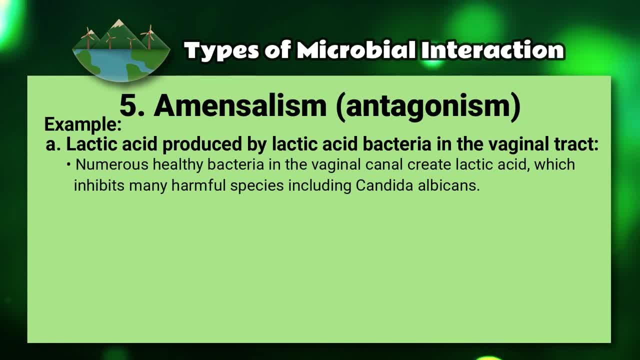 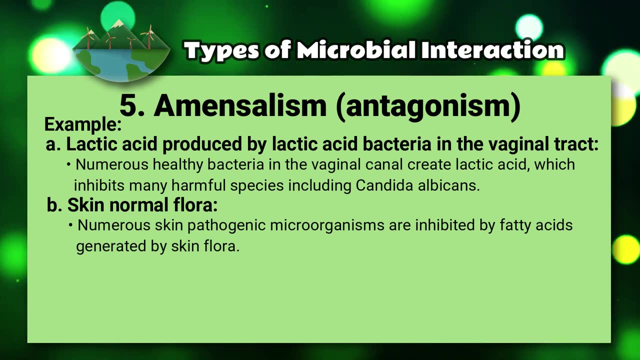 Numerous healthy bacteria in the vaginal canal create lactic acid, which inhibits many harmful species, including Candida albicans. 2. Skin normal flora. Numerous skin pathogenics in microorganisms are inhibited by fatty acids generated by skin flora. 3. Theobacillus thioxydate. 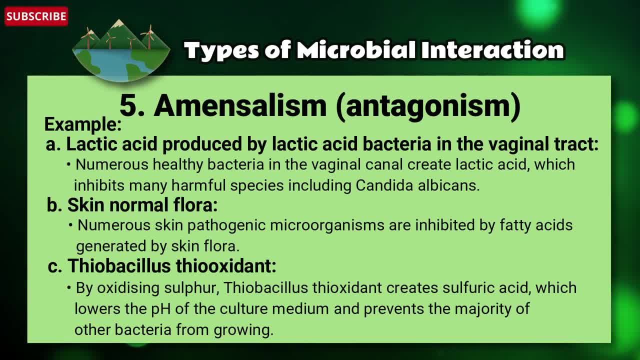 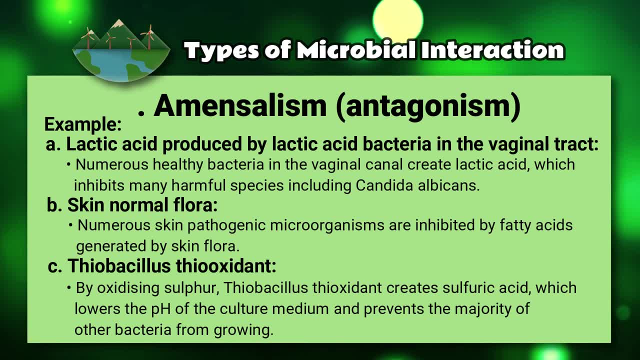 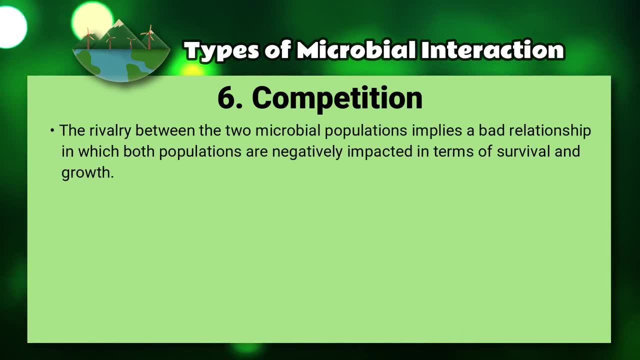 By oxidizing sulfur, theobacillus thioxydate creates sulfuric acid, which lowers the pH of the culture medium and prevents the majority of other bacteria from growing. 6. Competition- The rivalry between the two microbial populations implies a bad relationship in which both populations are negatively impacted. 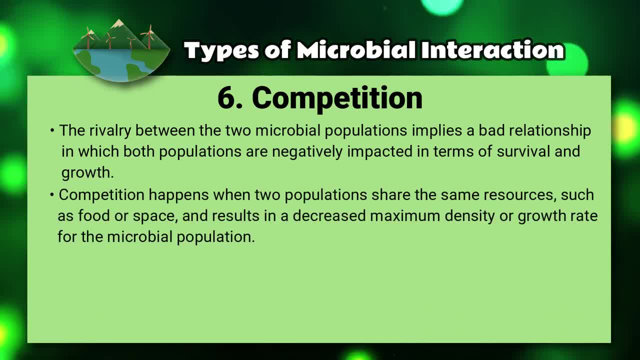 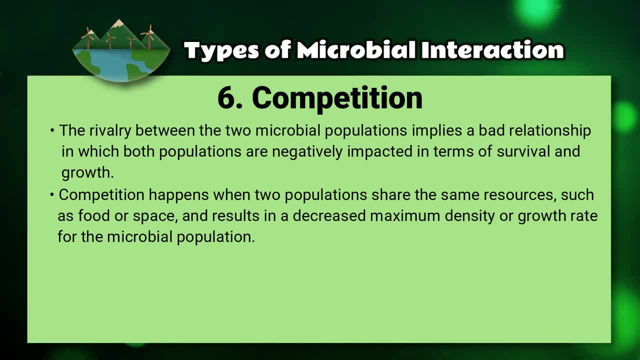 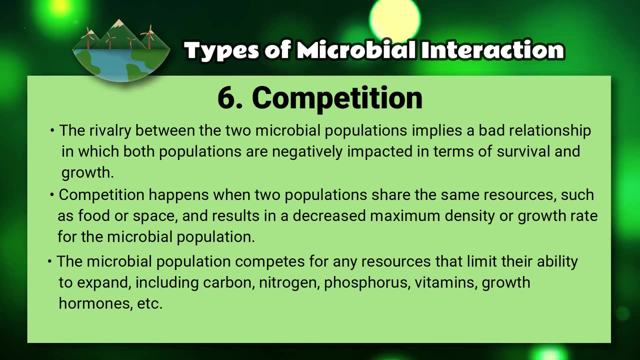 in terms of survival and growth. Competition happens when two populations share the same resources, such as food or space, which results in decreased maximum density or growth rate of the microbial population. The microbial population competents for any resources that limit their ability to expand. 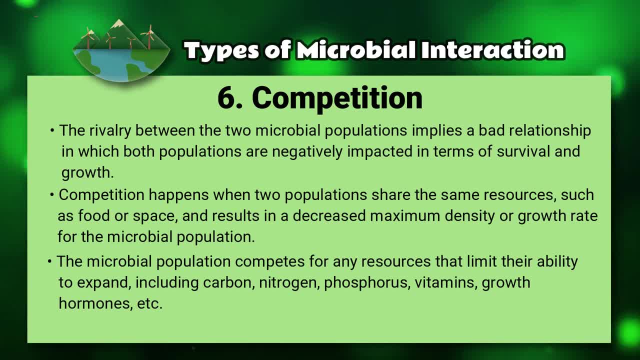 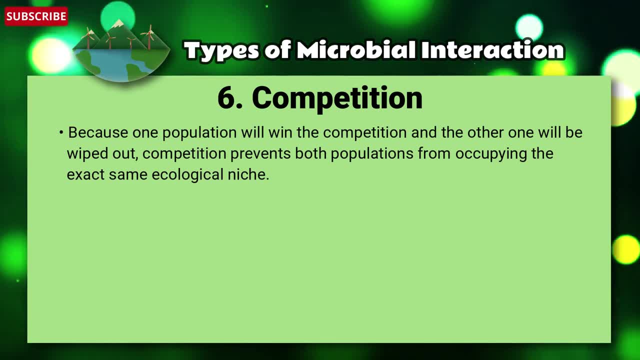 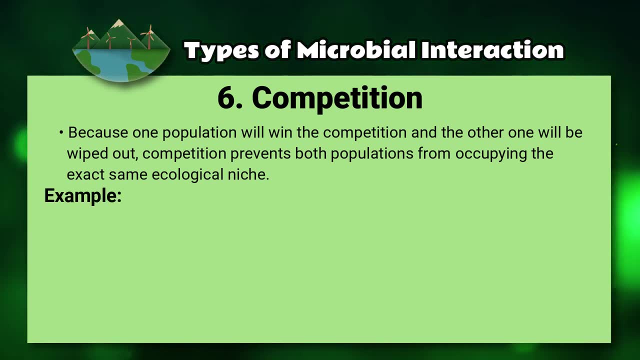 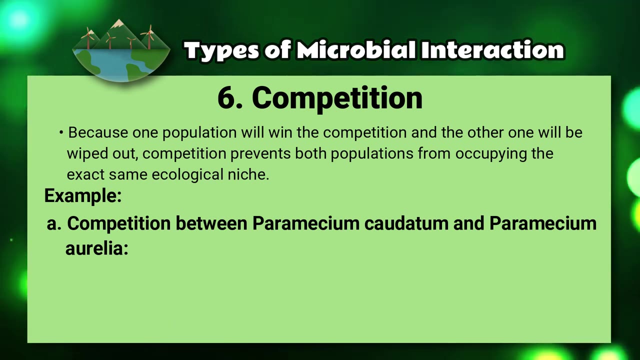 including carbon, nitrogen, phosphorus, vitamins, growth hormones, etc. Because one population will win the competition and the other one will be ripped out. competition prevents both populations from occupying the exact same ecological niche. Example of competition is Competition between Paramecium cantatum and Paramecium allurelia. 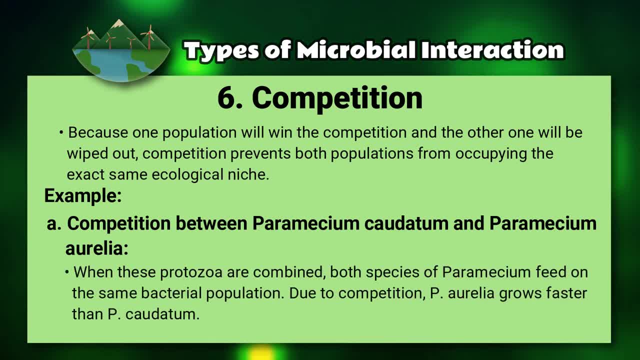 When these protozoa are combined, both species of Paramecium feed on the same bacterial population. Due to competition, Paramecium allurelia grows faster than Paramecium cantatum. Don't forget to support this channel by subscribing. 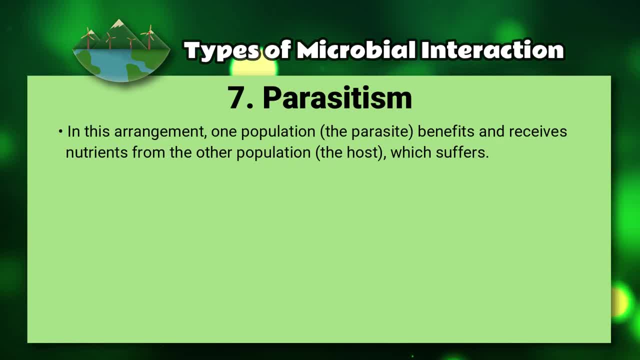 7. Parasitism. In this arrangement, one population- the parasite- benefits and receives nutrients from the other population, the host, which suffers. The population between a host and a parasite is defined by a considerable amount of time spent in touch. 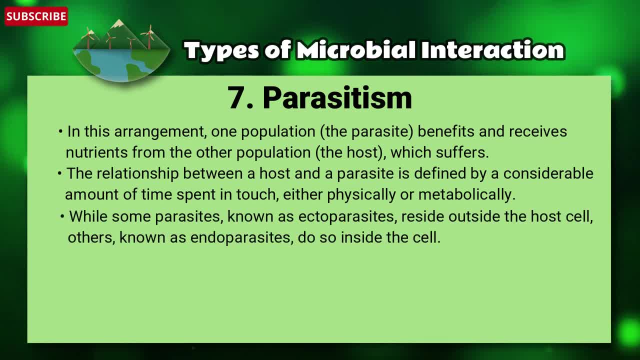 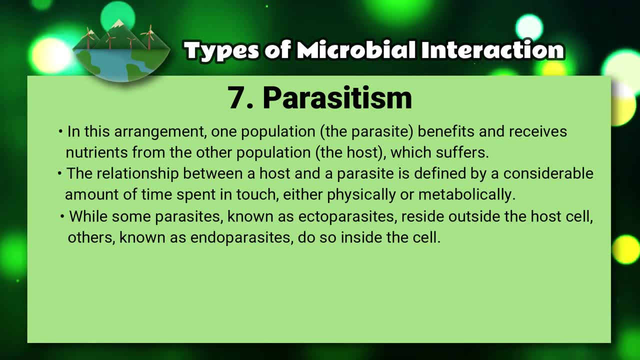 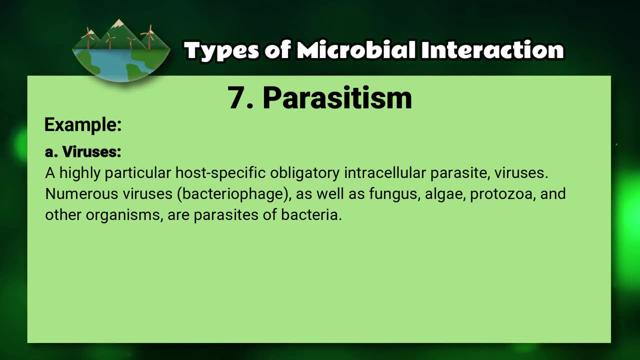 either physically or metabolically. While some parasites known as ecoparasites reside outside the host cell, others, known as endoparasites, do so inside the cell. Examples are: 1. Viruses, A highly particular, host-specific, obligatory intracellular parasite. 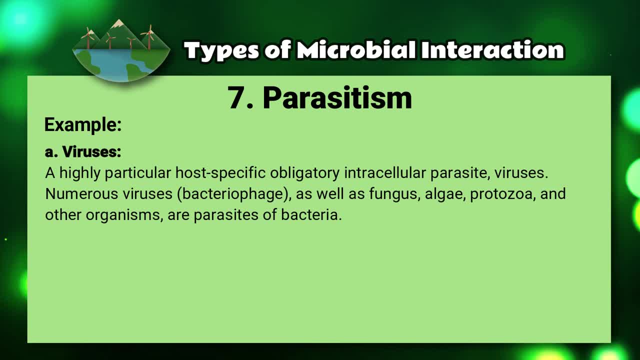 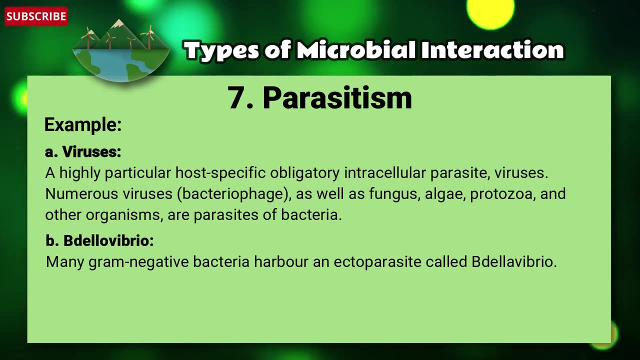 viruses- Numerous viruses, bacteriophage, as well as fungus, algae, protozoa and other organisms, are parasites of bacteria. 2. Bidellovabria: Many gram-negative bacteria harbor on ectobacterium called Bidellovabria. 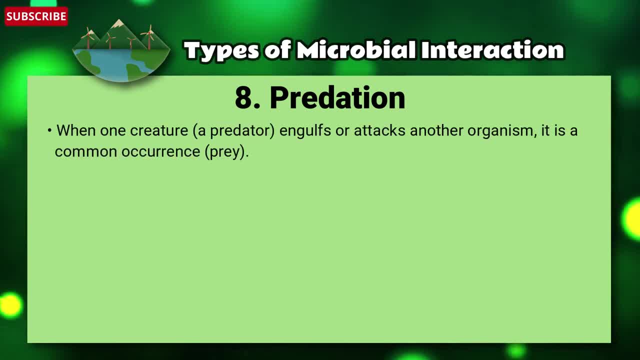 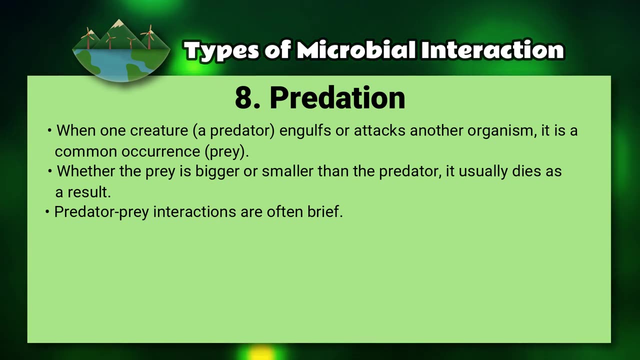 3. Predation: When one creature, a predator, engulfs or attacks another organism, it is a common cocrans. When the prey is bigger or smaller than the predator, it usually dies as a result. Predator-prey interactions are often brief. 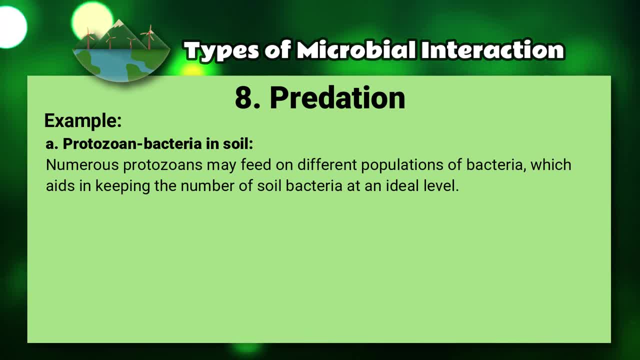 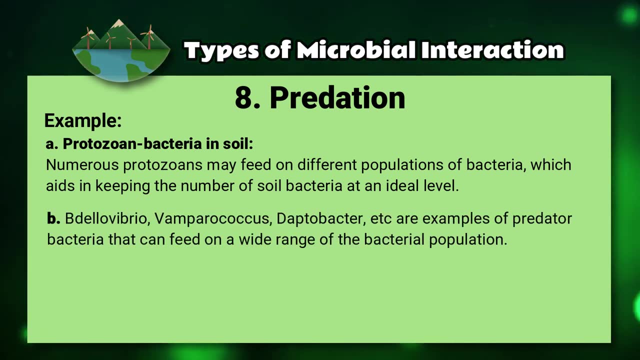 Examples of predation are: 1. Protozoan. Numerous protozoans may feed on different populations of bacteria, which aids in keeping the number of soil bacteria at an ideal level. 2. Bidellovabria- Baryococcus Depthobacter.